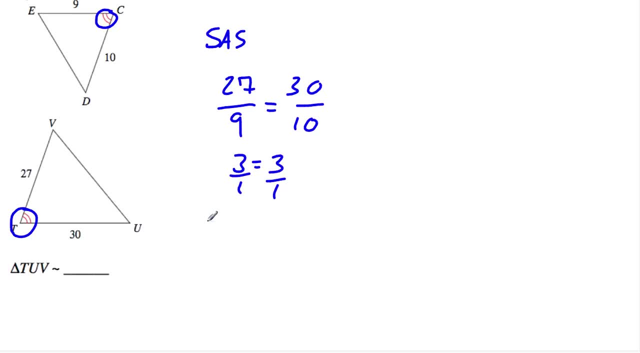 These are the same proportion. This is a scale factor. 3 to 1 equals 3 to 1.. Because these sides are proportional, the angles are congruent. I have side angle side, So now I have to write a similarity statement. So I have the triangle TUV. TUV is similar. 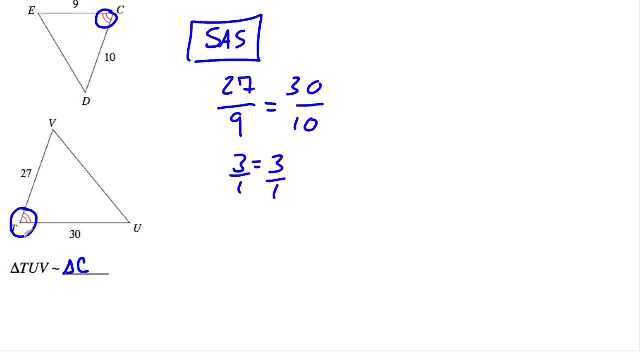 to triangle. Well, T again is C and here U is going along this long side. So the long side here is D and I wrap up with E. So that's side, angle side, Again showing two sides are proportional and the angle in between is congruent. I could also have this where no sides are given. Remember, if we have 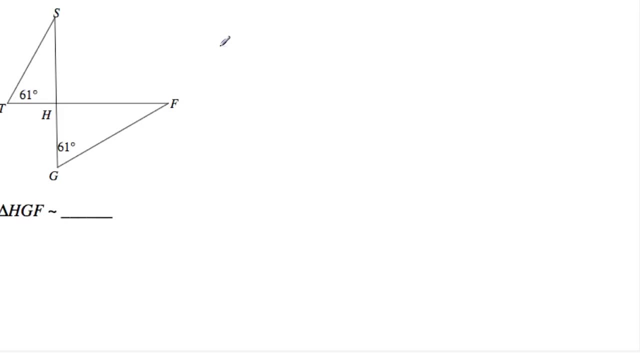 side side, side side angle side, and then angle angle. no sides are given. chances are you're going to be using angle angle. Actually, we can see here that these two angles are congruent. Measures are given, And then these two are also congruent because they 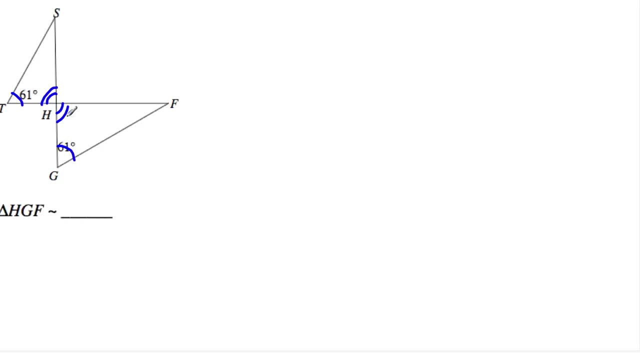 are vertical angles. So if I've seen that these two angles are congruent, that's it. These two triangles are similar because of angle angle. So triangle HGF is similar to triangle HTF. Okay, Okay, Okay, Okay. 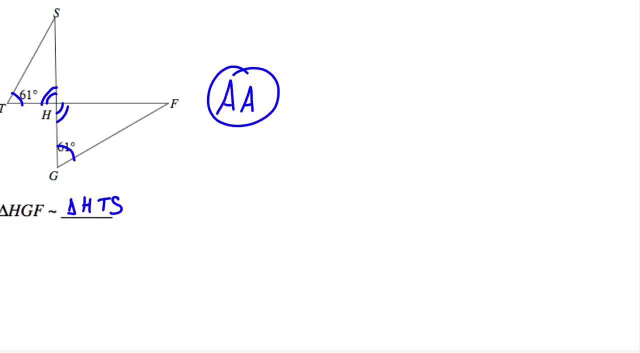 Okay, Okay, just like that, quick and easy. and then finally we could have this side side side. so no angles are given here, but we're probably gonna be looking at side side side. if I can show that all the corresponding sides are proportional, that means that the triangles are similar. so 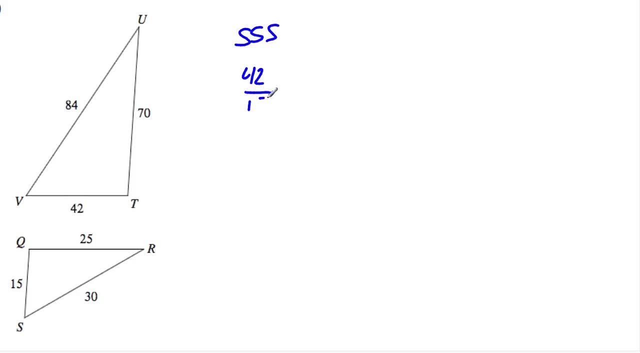 I could do 42 to 15. that's a short side. there should equal 70 to 25, and then that should equal 84 to 30. again, with all of these we can, it might be easier to use a calculator for you we can find. 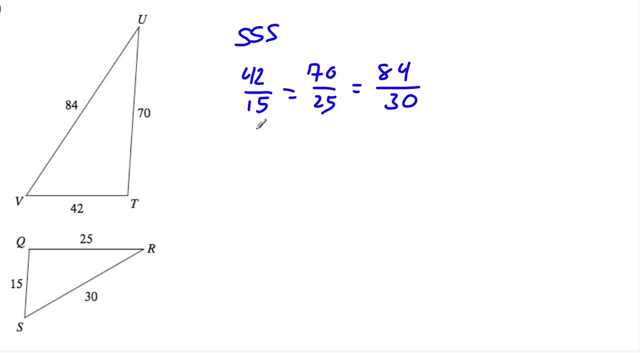 common factors. we can reduce. but you know what I'm not gonna have you. I don't require you to do that. so if you can get, hey, put this my calculator 2.8, that's perfectly fine. as long as we're getting getting the concept and as I put all of these into my calculator and I can't see this. but if you try,